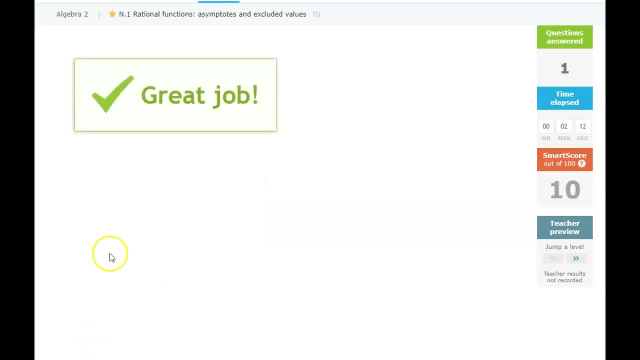 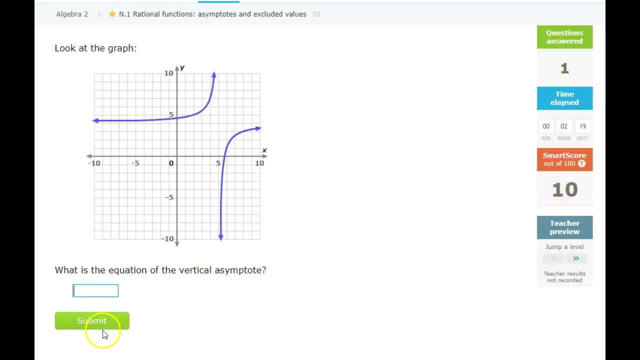 Y equals four. What is the equation of the vertical asymptote? So again, we're looking up and down. So our vertical asymptote is at x equals five. What is the equation of the vertical asymptote? So we're going to come over to the left here and see how the curve is approaching not one, two, So it's approaching actually negative two. 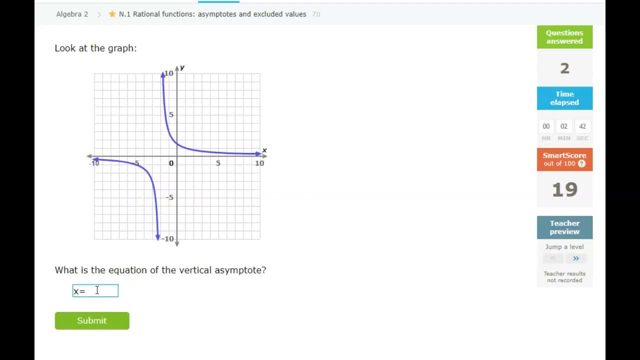 So we're going to say x is equal to negative two. What is the equation of the horizontal asymptote? So again, we're looking side to side. We're looking where the curve is approaching, but not touching The curve is approaching. y is equal to zero. 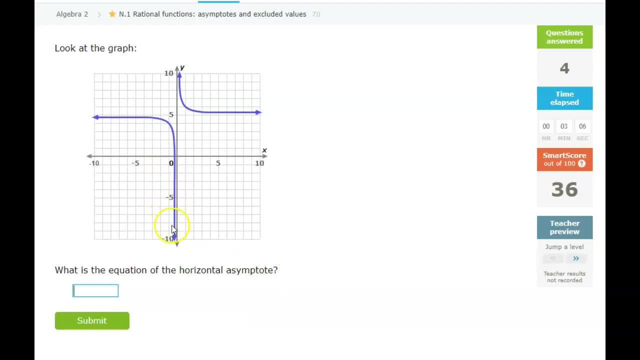 What is the equation of the horizontal asymptote? So again, we're looking at the left, here at four. So we're going to say x is equal to negative two. So we're going to say y is equal to negative two. What is the equation of the horizontal asymptote? So again we're looking at the left, here at four. So it's approaching negative two. 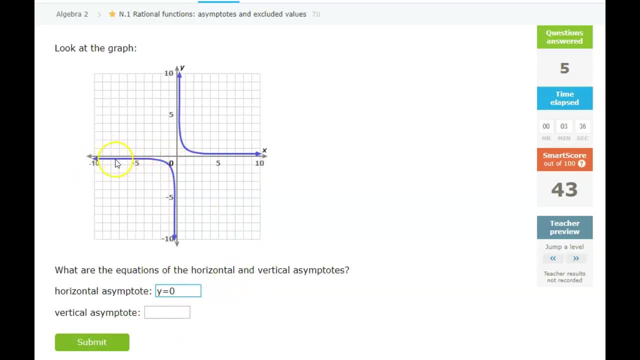 because the curve is approaching 0, but we'll never touch it. Our vertical asymptote- you see the curve here approaching, So you're looking up and down. It's approaching the y-axis, So it would be x is equal to 0.. 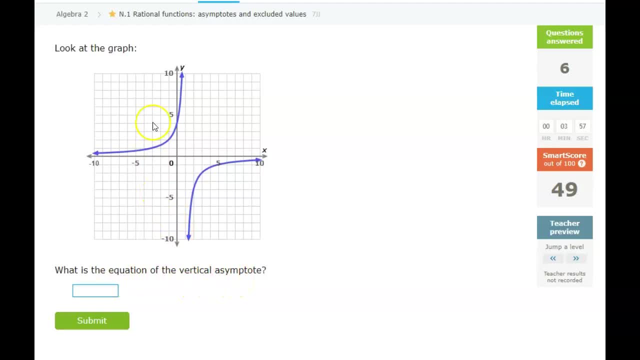 What is the equation of the vertical asymptote? So again, we're looking at the curve as it extends to positive infinity and negative infinity, and we see that the curve is approaching x equals 1.. What is the excluded value for this function? 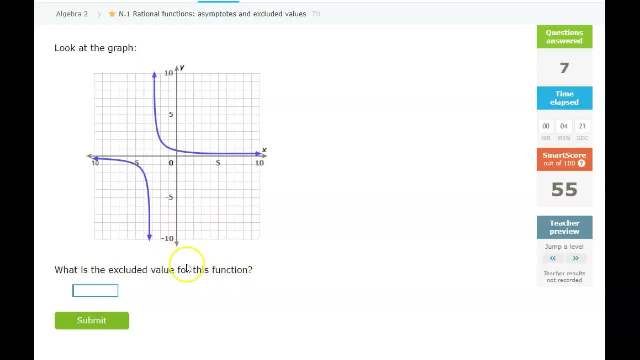 Now this time they're not asking us what's the equation of the line, They're saying what number do you not include? So here we see that the line Y, or the curve, is approaching negative 3.. So the excluded value would be negative 3.. 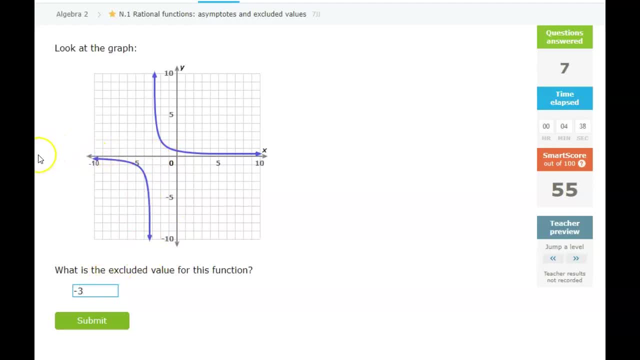 So if we were writing our domain, we would say: Our domain includes Or does not include. I'm sorry, Infinity is an idea, not a number, So we would have open bracket. Let me see if I could draw it here. 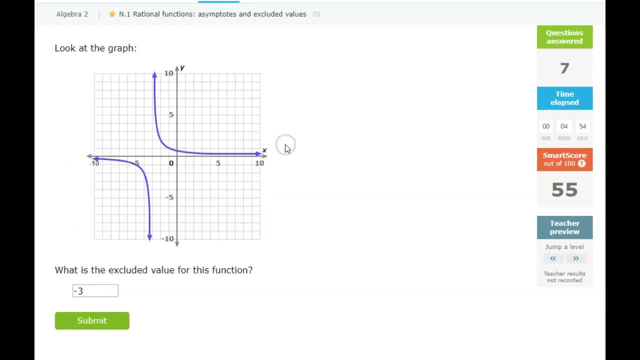 We would have Interesting. I thought I could draw. There we go Freehand, that looks good. Let's do blue. No, Let's do Yellow. won't work. Let's do green. No, Let's do purple. 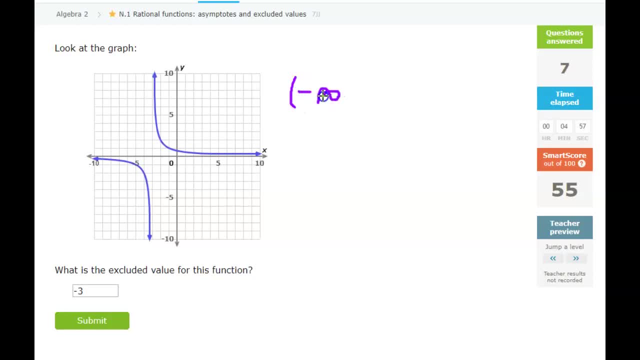 Yeah, we like purple. So negative infinity Comma, And then it's approaching Negative 3.. So this is our domain we're talking about, Or from negative 3 to positive infinity. Close the parentheses. The parentheses just mean that that value is not included. 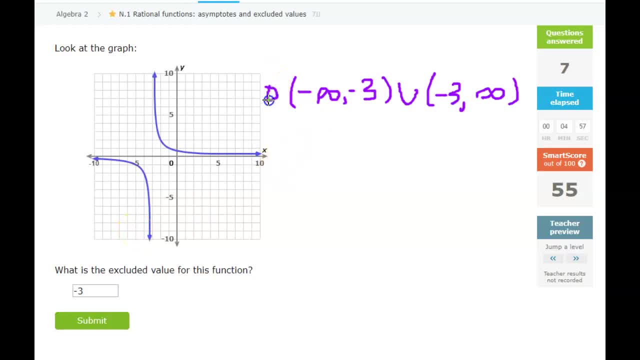 And then. so this would be the domain Arrange, And I probably won't do this again, so make sure you pay attention- Is negative infinity, Negative infinity to 0, union, Or you could say, or From 0 to positive infinity. 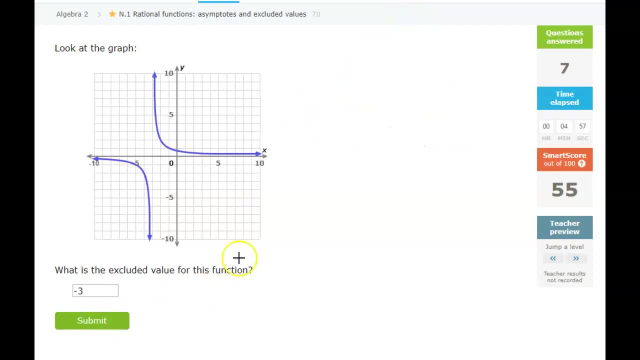 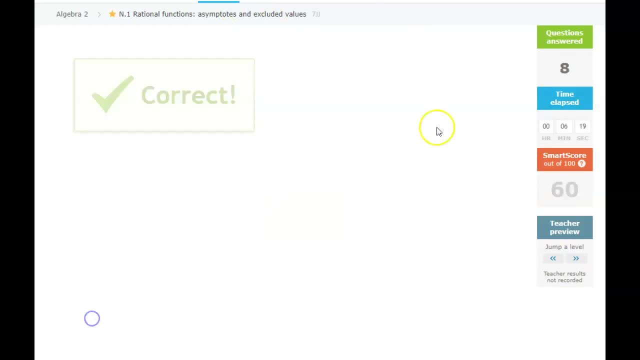 So now I'm going to erase it all, Because I don't know what it's going to do now, Because I've never used that before. I just thought it would be fun. So let's take that off And we're going to skip it. 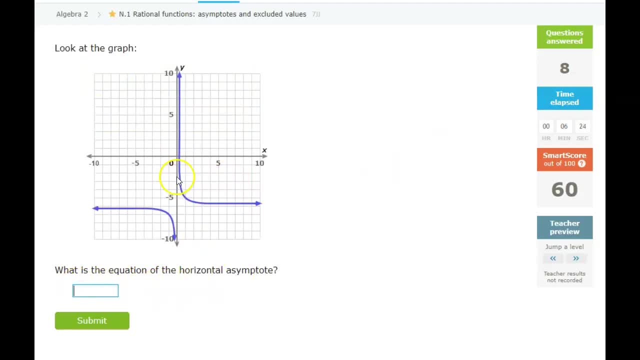 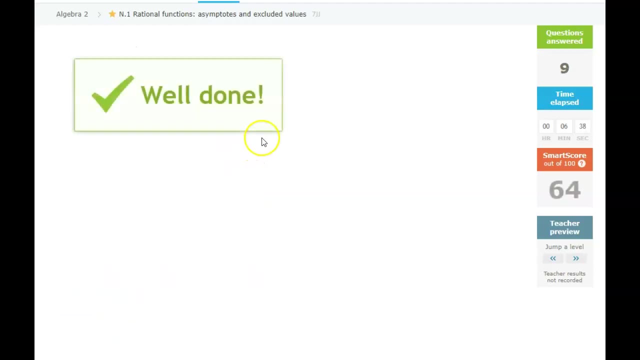 So what is the equation of the horizontal asymptote? Well, the curve Is approaching the line that would go across the y axis, And so a horizontal asymptote would be: y is equal to negative 6.. What is the equation of the vertical asymptote? 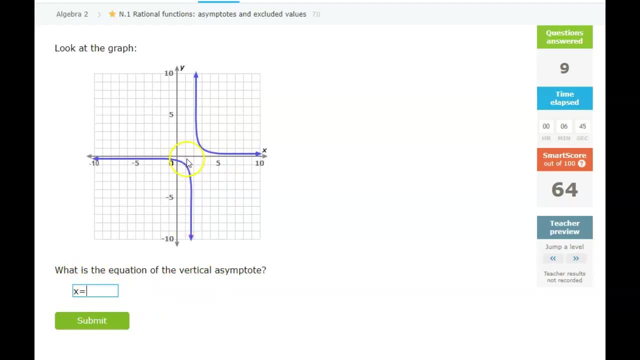 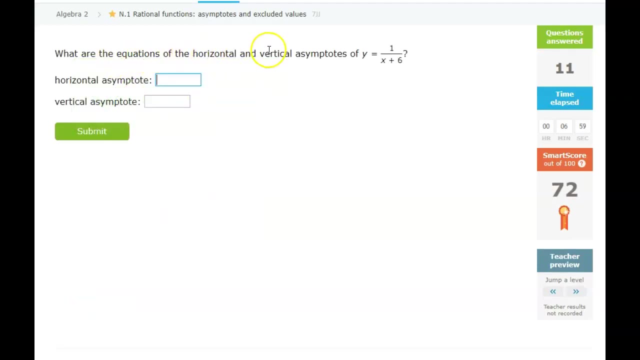 Well, we know, vertical is x equals, And it is approaching. 2. What is the excluded value? Well, the excluded value would be negative. 4. What are the equations of the horizontal asymptote and the vertical asymptote? Now, remember, the vertical asymptote is found here, in the denominator.